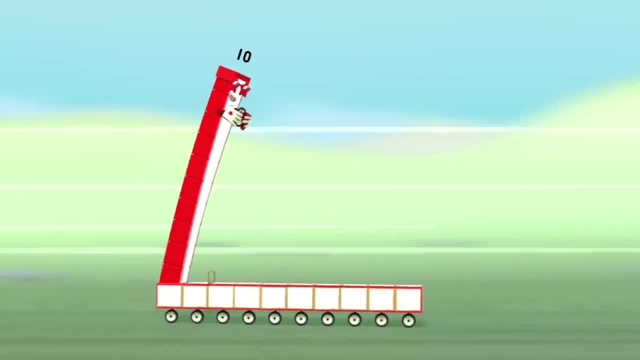 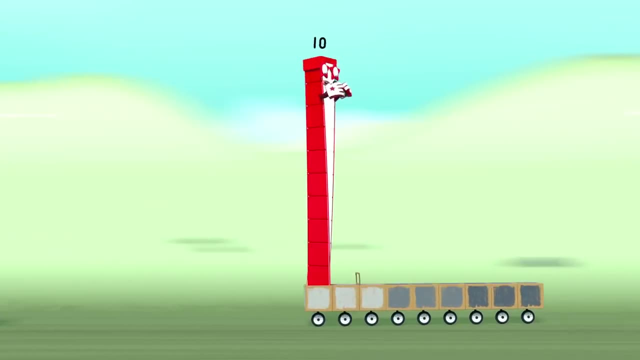 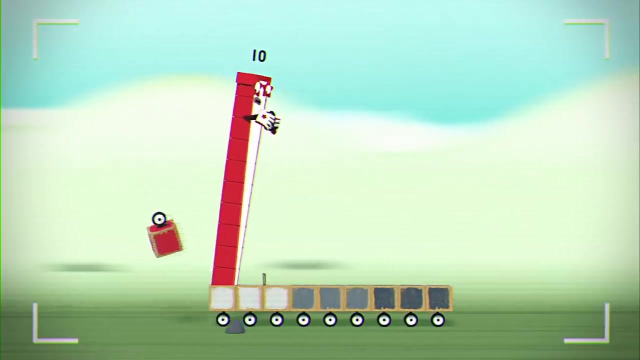 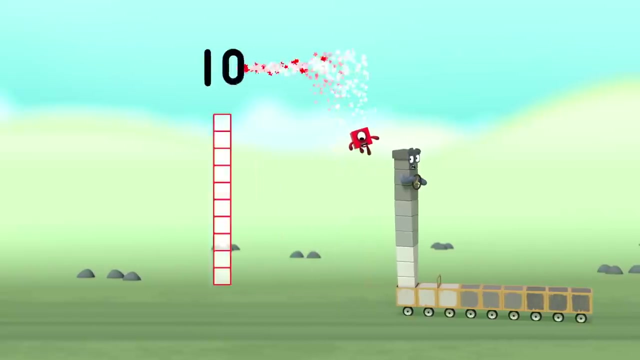 10 is in the lead. With 10 wheels, she seems unbeatable. But wait, She's lost a wheel. Let's see that again in slow motion: 10 wheels minus 1 wheel equals 9 wheels left. 10 minus 1 equals 9.. 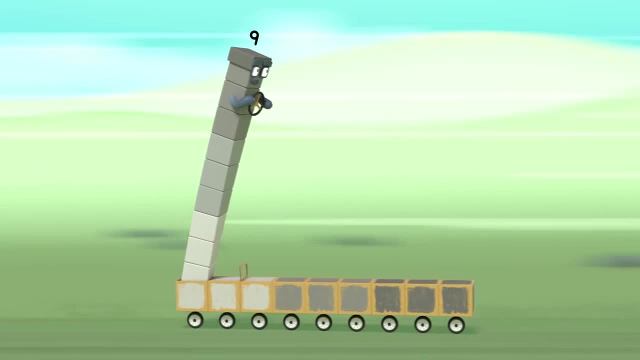 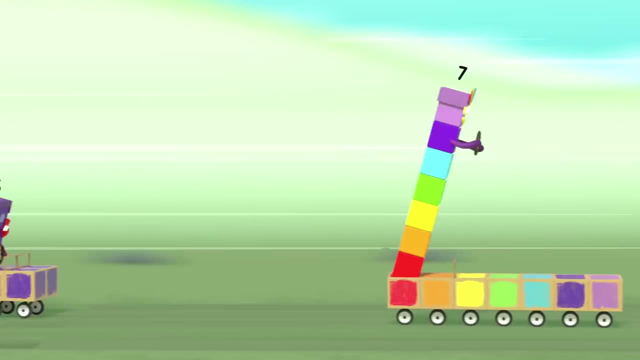 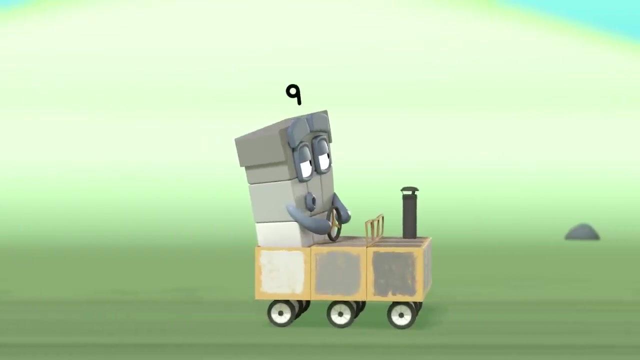 Hey Go, 9!. 10 is out of the race as 9 takes a surprise lead. Nice day for it. And what makes it really surprising is that 9's in last place too Well, next to last, keep pedalling, Ron. 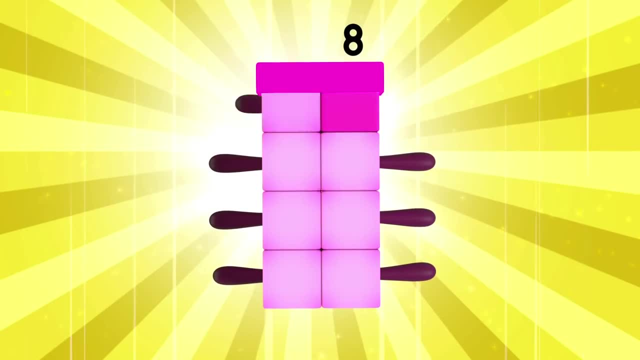 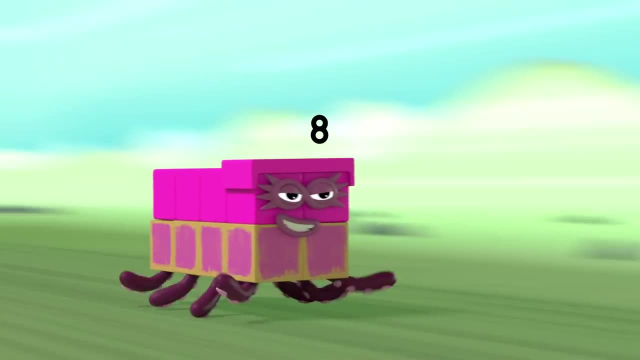 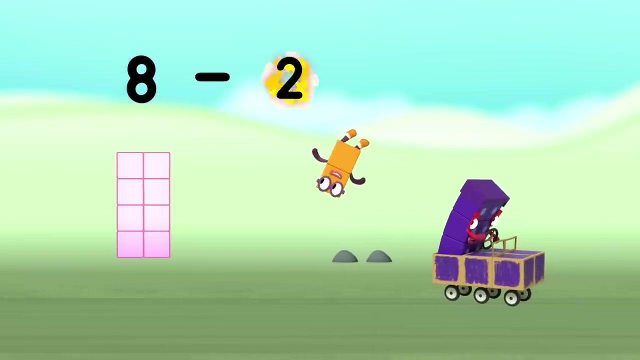 Octoblock race 1,, 2,, 3,, 4,, 5,, 6,, 7, 8, race. It's in trouble. Those two quadroblocks are about to go. 8 minus 2 equals 6.. 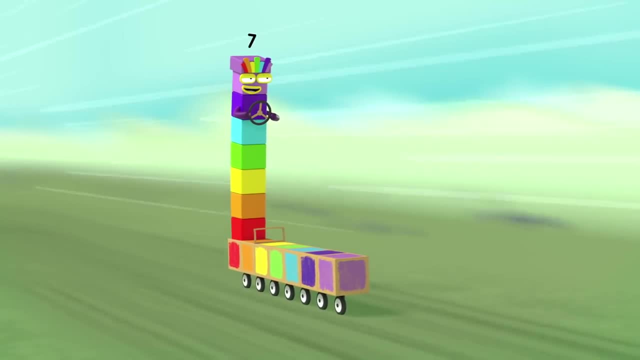 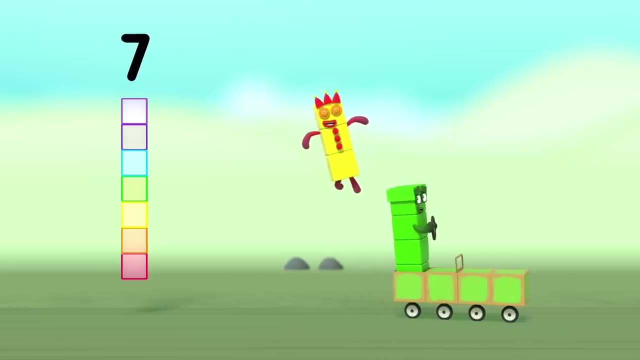 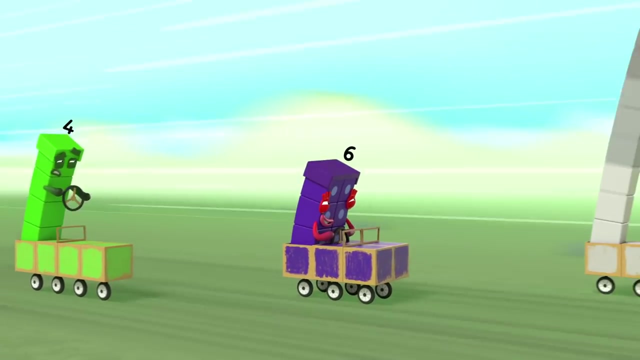 Look out, Phew, That was lucky. 7 minus 3 equals 4.. Four-wheel drive: Yay, Yay, Yay, Yay. 6 has caught up with 9 as they enter the double dipper. 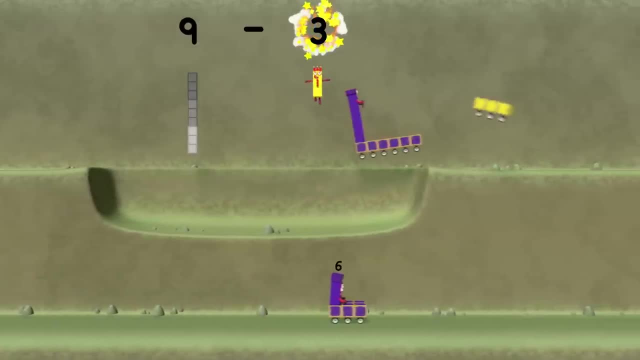 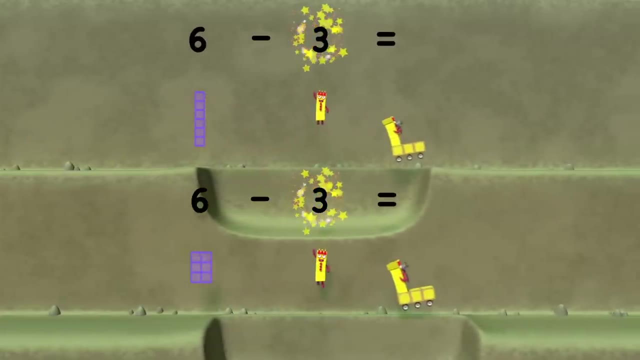 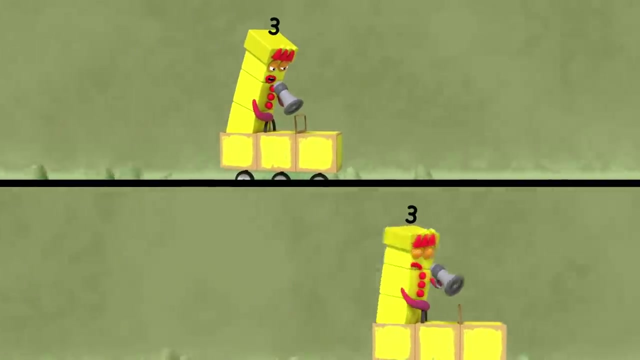 Mind that dip 9 minus 3 equals 6.. And the double dips, Six minus three equals three. And what a cliche for nine. Six couldn't get fine there. Do you mind? I'm commentating here. No, I'm commentating. No, I am. 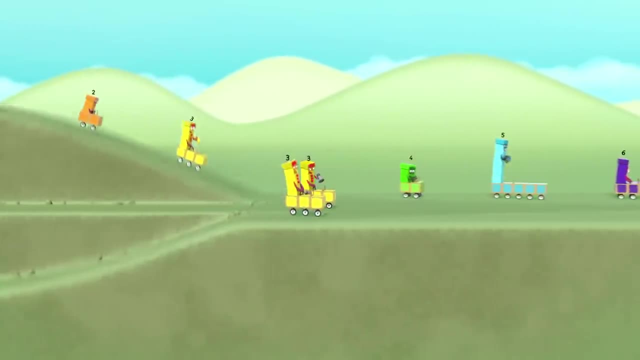 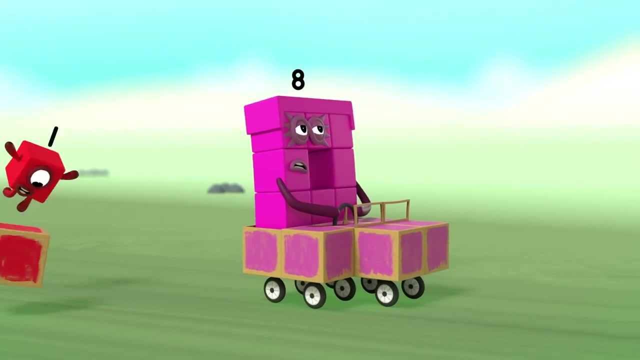 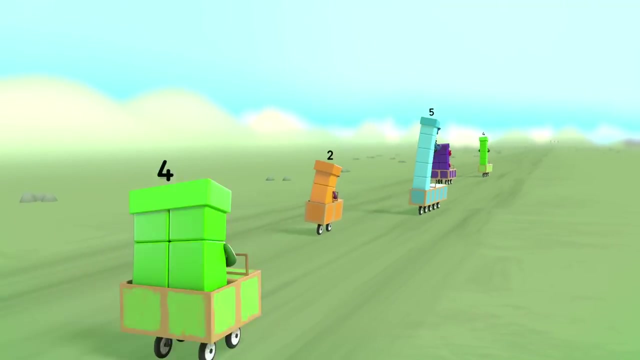 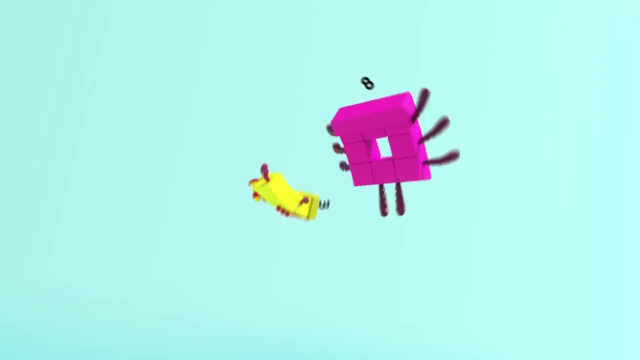 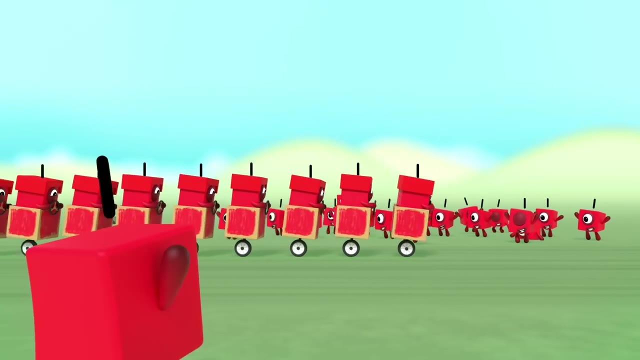 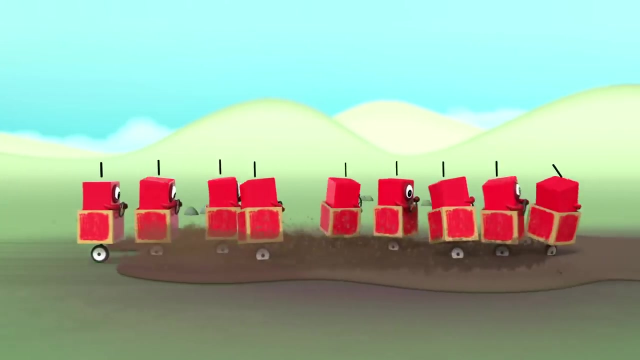 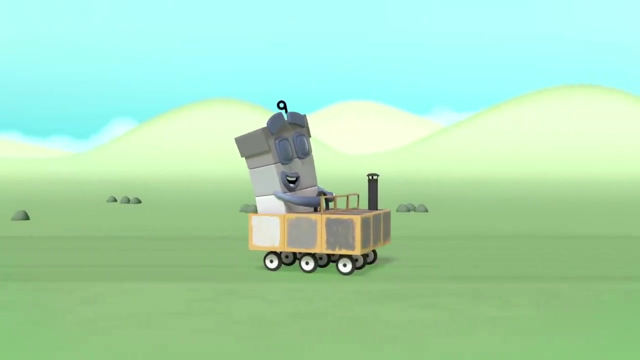 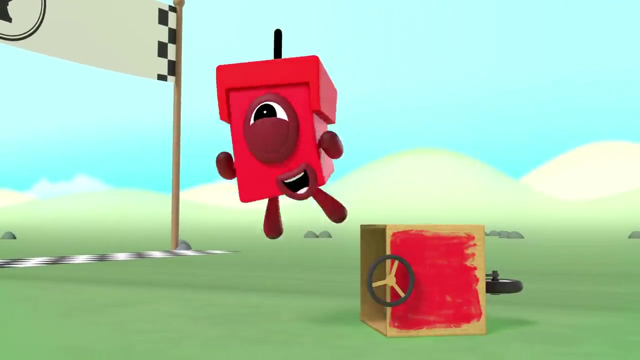 Uh-oh, Uh-oh, Uh-oh, Uh-oh, Uh-oh. And it's one in the lead, Followed by one, But here's one coming up on the inside. Nine wolves equals Nine. Nice day for it, I'm first. Oh yeah, Woo-ho-ho-ho-ho. 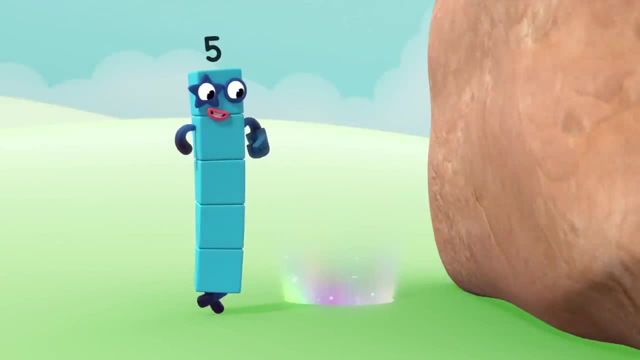 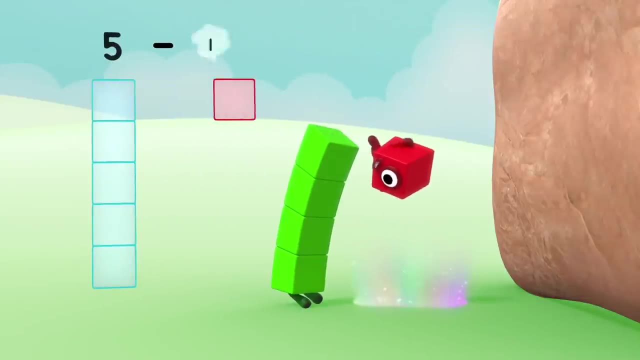 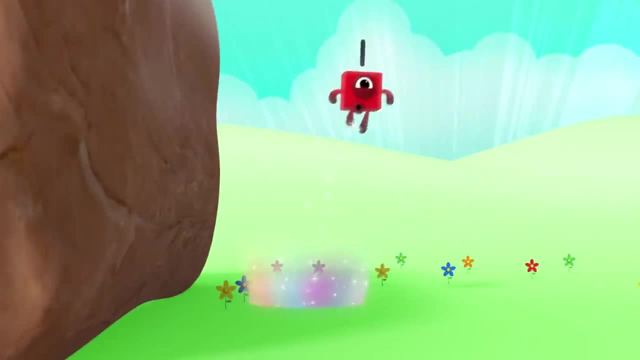 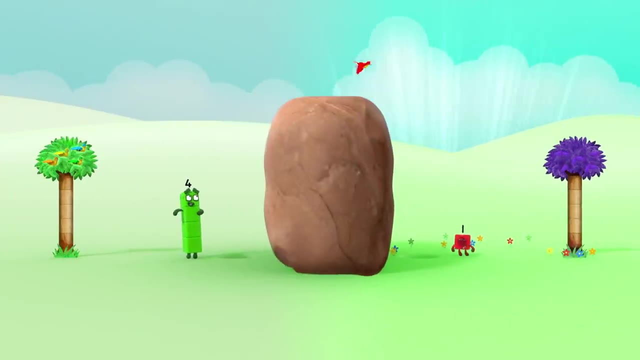 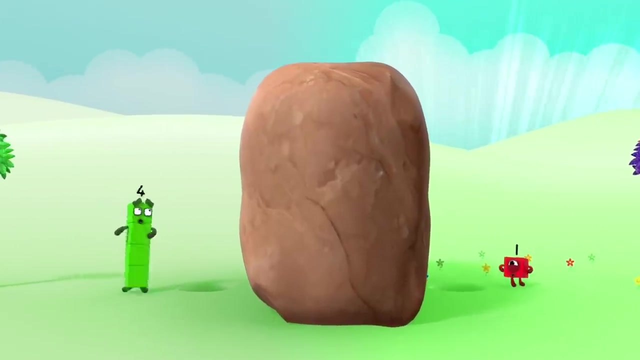 My head fell off. Where did it go? Woo-hoo, I have won. That was fun. Now I am four, and here I am. I am one, here I am. What a wonderful day to be alive. But where, oh, where, oh, where is five? 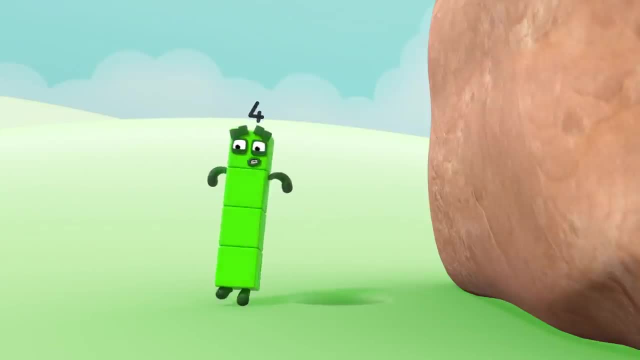 Five is gone. where did she go? Is she alright? I do not know. Is she here? Is she there? I must keep looking everywhere. What is that silly sucking sound? A giant hole so big and round? Why is it there? I do not know. 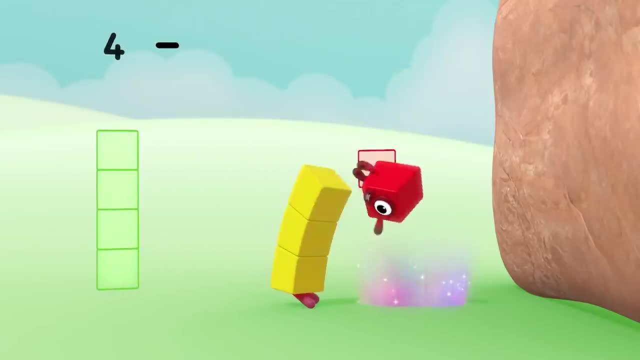 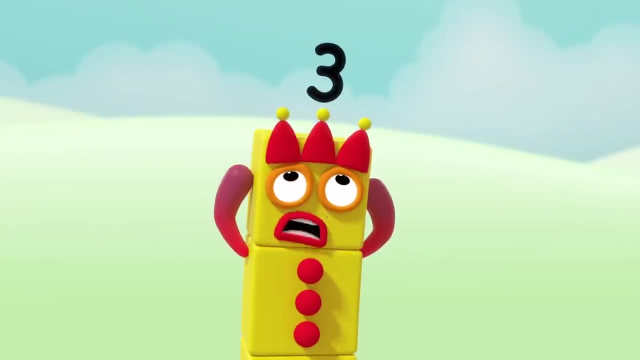 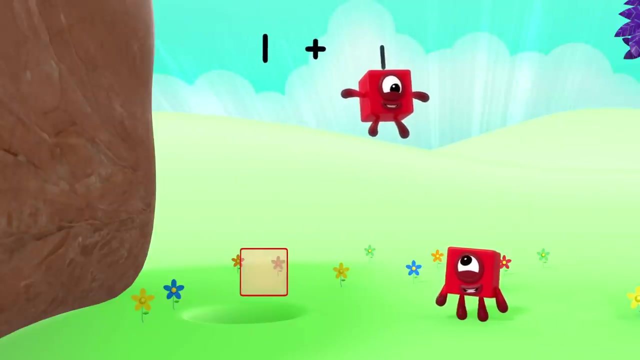 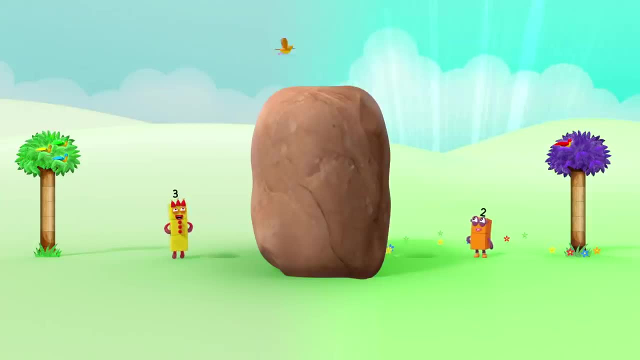 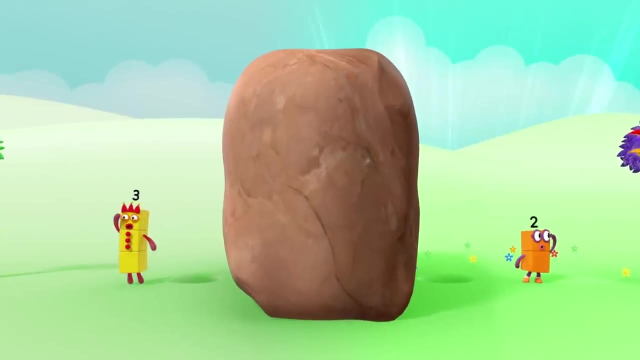 I just got bigger, did you see? Now I am three and here I am. Now I am two and here I am. What a wonderful day to be alive. But where, oh, where, oh, where is five? I was five, then four, then three. 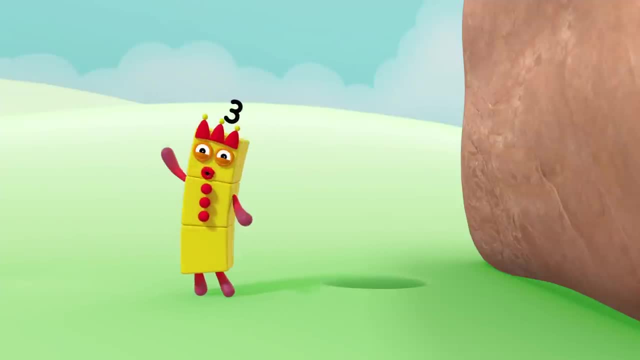 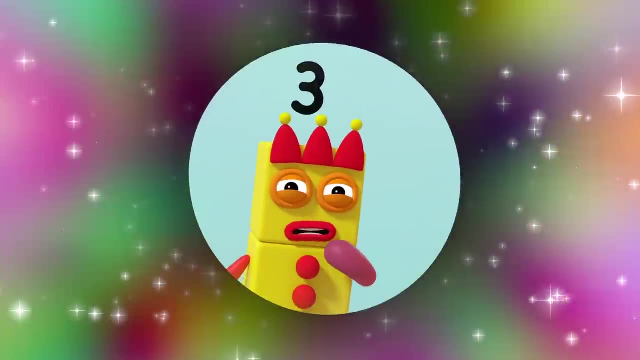 Someone has played a trick on me. I do not mind at all. you see, Three is who I want to be. What is that silly sucking sound? A giant hole so big and round. Why is it there? I do not know. I wonder what is down below. 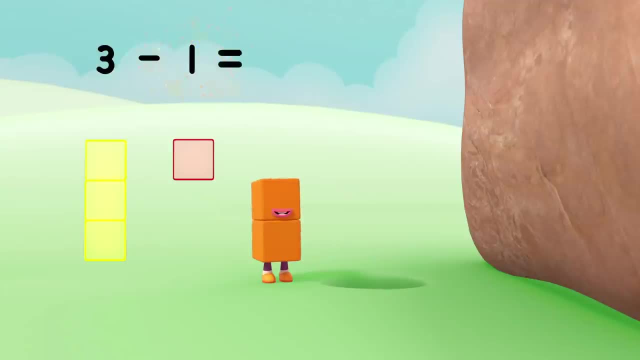 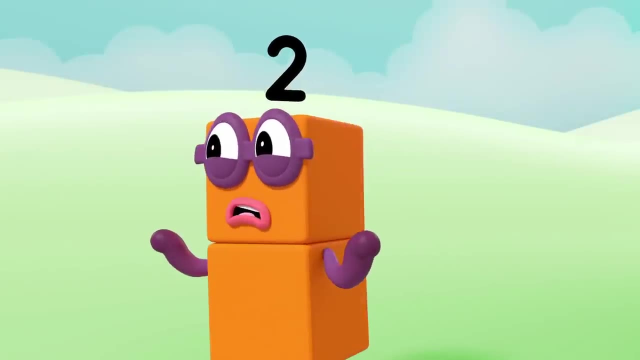 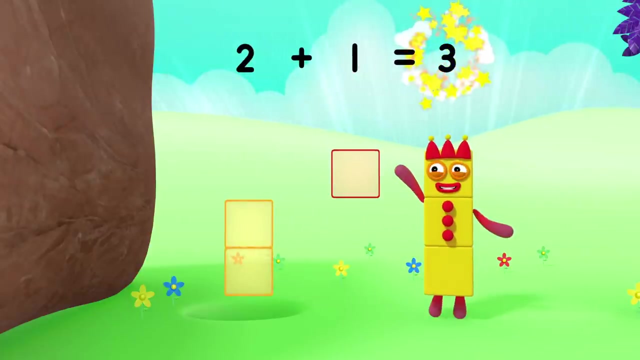 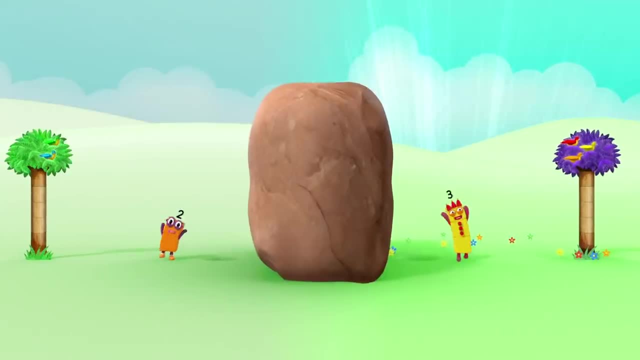 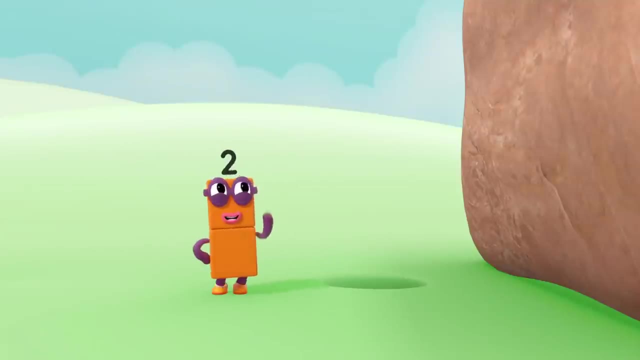 Now I am two, and here I am. Now I am three and here I am. What a wonderful day to be alive. But where, oh, where, oh, where is five? I wonder where the ones will go. I think I've got it now, I know. 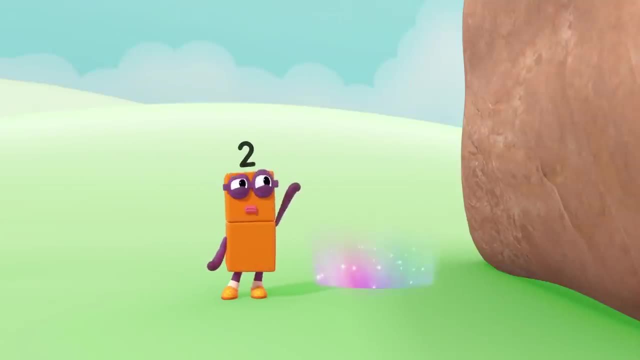 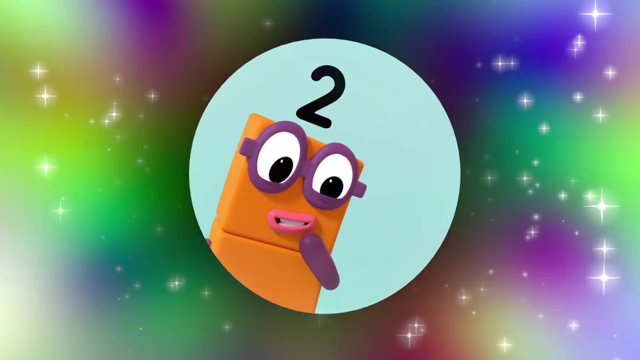 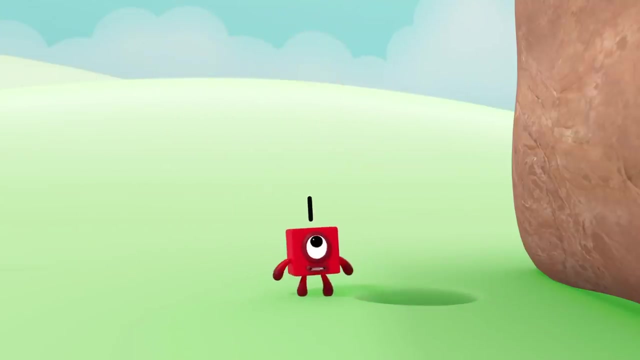 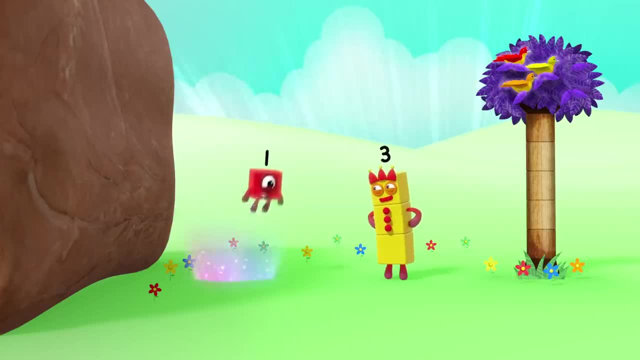 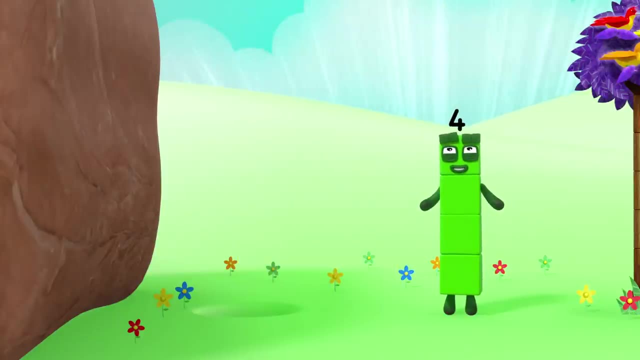 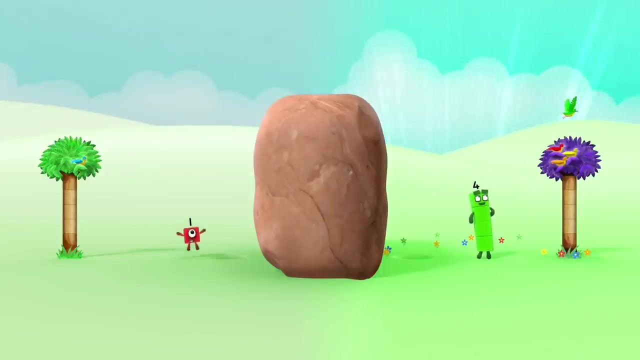 My head fell off. where did it go? I am one. that was fun. Three Plus one Equals four. What is happening to me? I just got bigger, did you see? Now I am one, and here I am. Now I am four, and here I am. 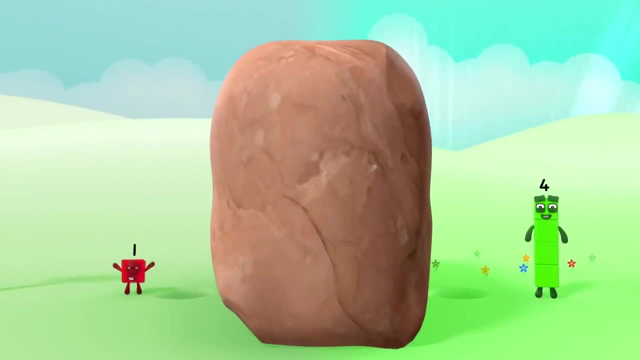 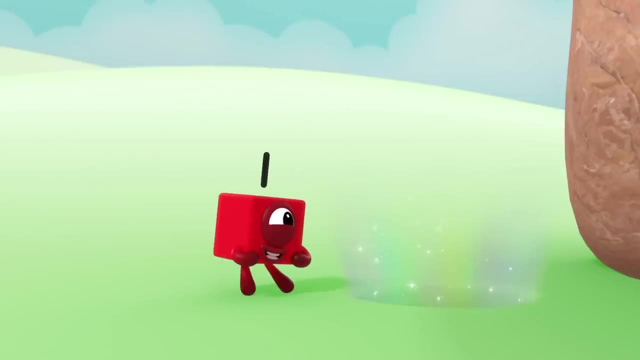 What a wonderful day to be alive. But where, oh where, oh where? is five, Five, four, three, two, one. Someone's having lots of fun. Now I know where five will be. Four is waiting there for me. What is that silly sucking sound? 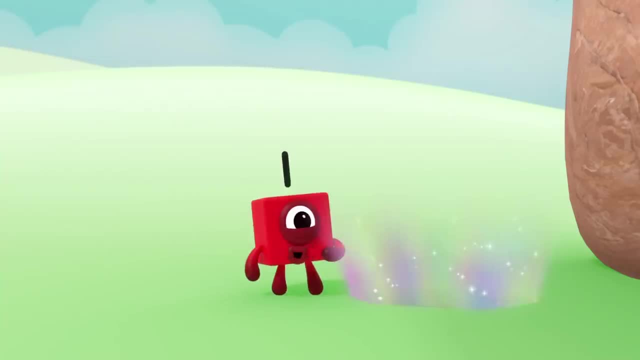 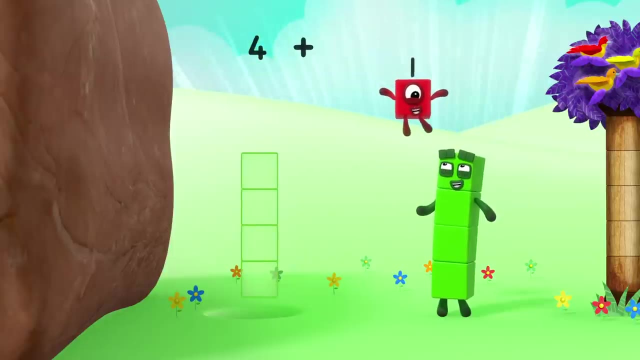 A giant hole so big and round. Why is it there? I think I know. I think I know what's down below. I am one. that was fun. Four Plus one Equals five. What is happening to me? I just got bigger, did you see? 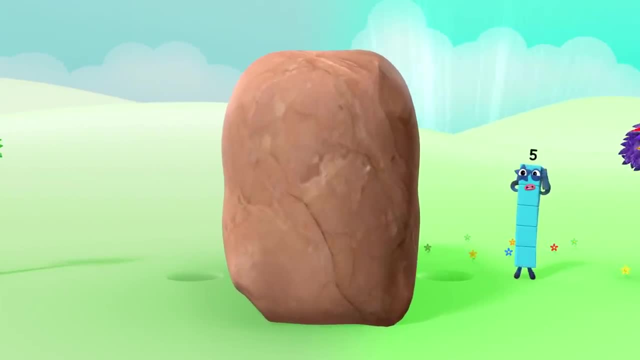 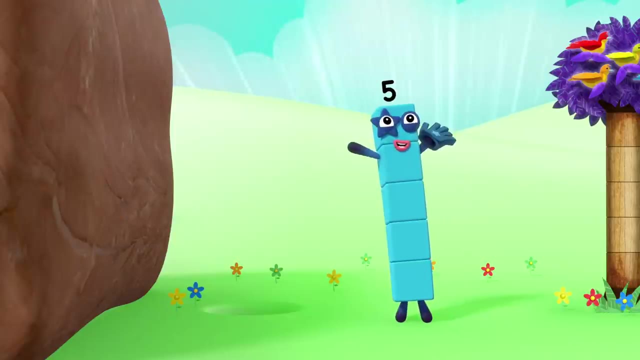 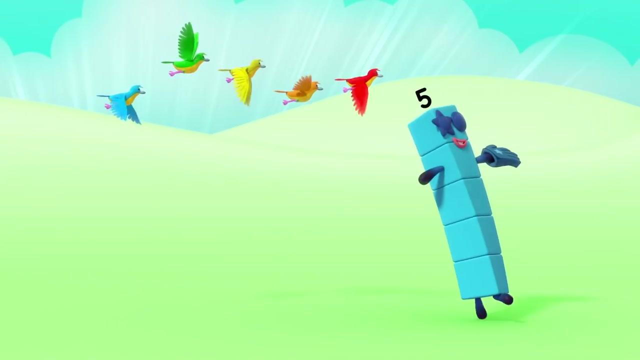 What a wonderful day to be alive. But where, oh, where, oh, where is five? Here I am, and I am five. What a wonderful way to arrive. One, two, three, four, five. What a brilliant, amazing, fantastic, terrific and wonderful day to be alive. 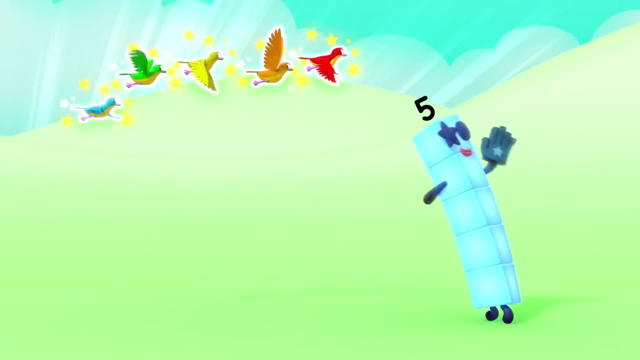 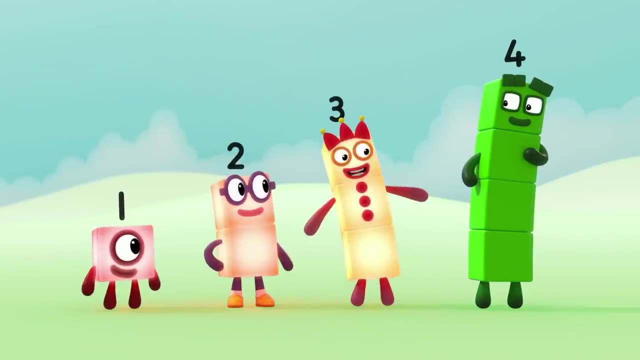 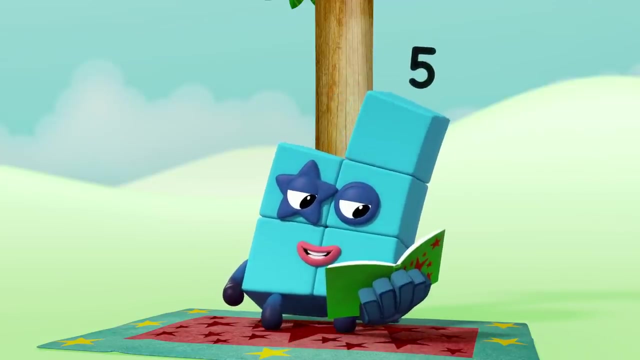 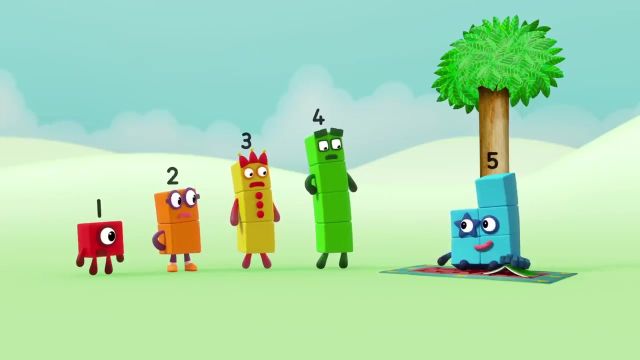 One, two, three, four, five. Hello, We're playing hide and seek. Want to join in? I would absolutely love to You hide and I'll seek. You won't find us sat there, Oh, will I not? now? I'm good at this game. 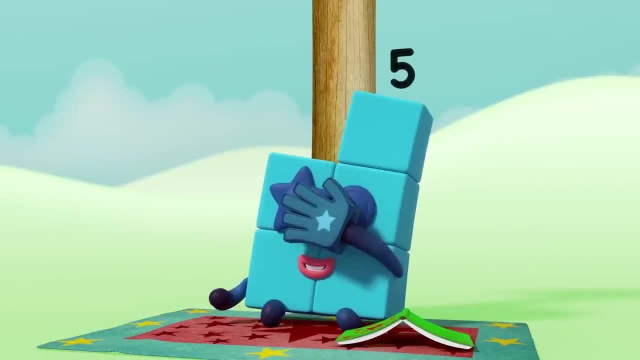 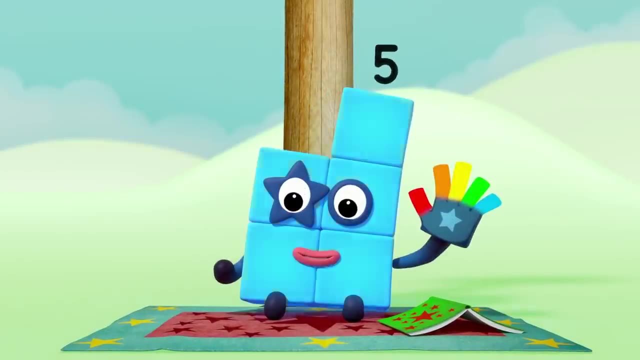 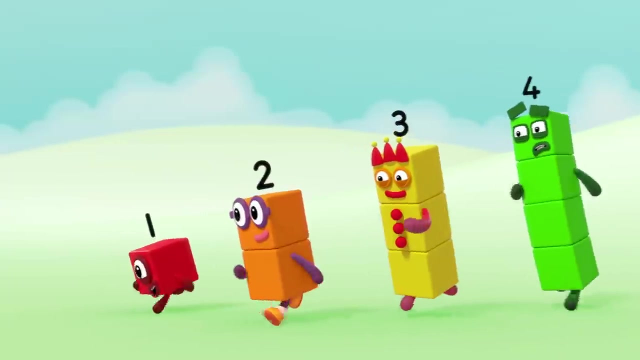 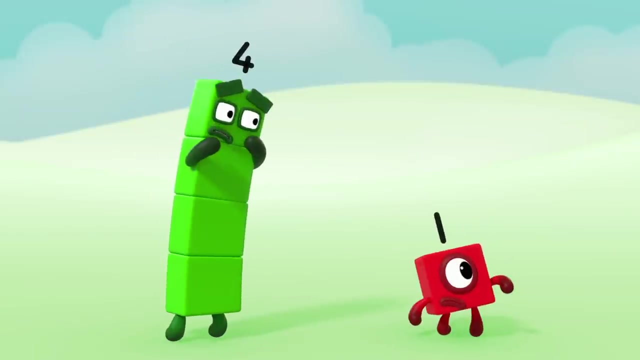 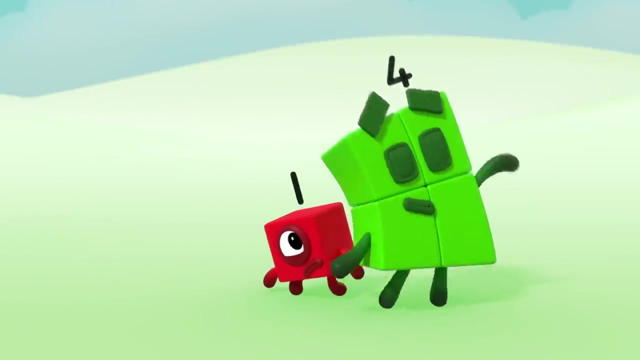 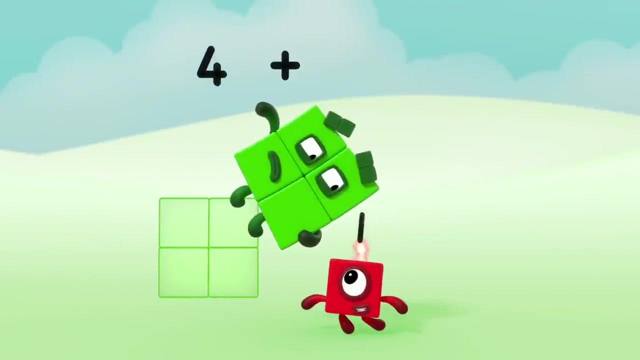 I'll find you and point you out. One, two, three, four, five. Ready or not? here I Get on with my book. Hey, hide behind me. Where can I hide? I know behind you. Four Oops. Four Plus one Equals five. 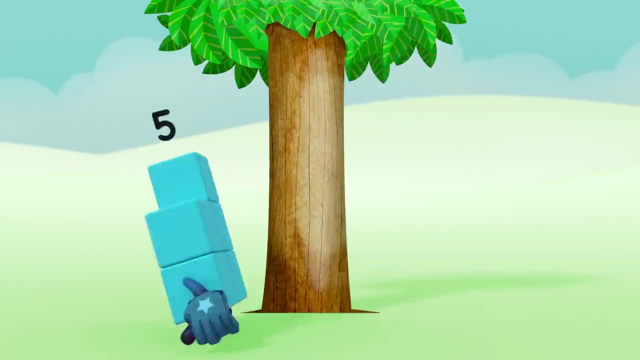 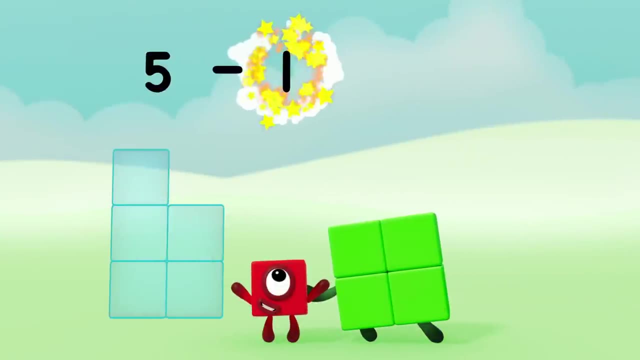 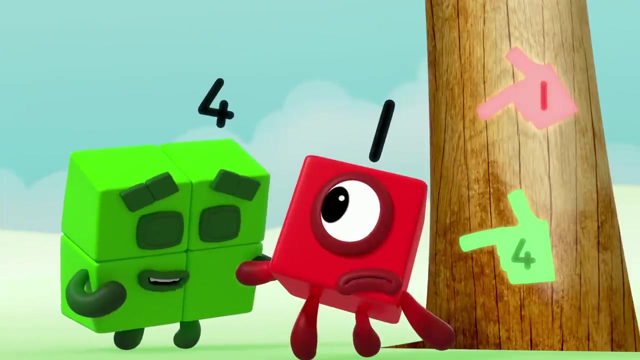 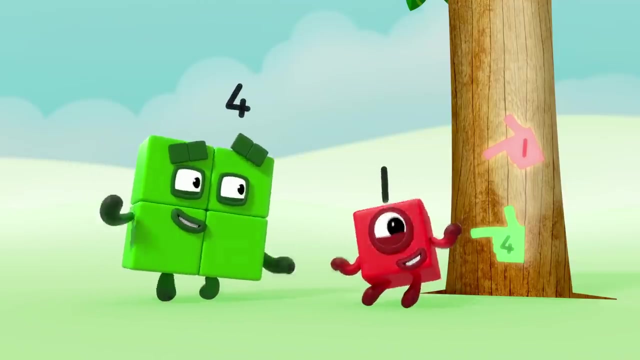 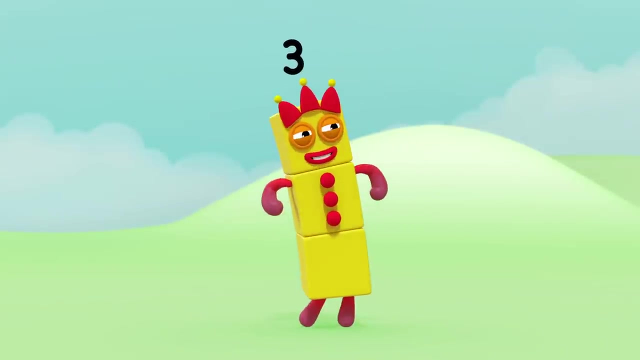 Ready or not, here I come. Find you four, find you one. Five minus one Equals four. Look, five, said you'd point us out. Five was right here. How I am Three Master of Disguise. Ah, Shhh, Shhh. 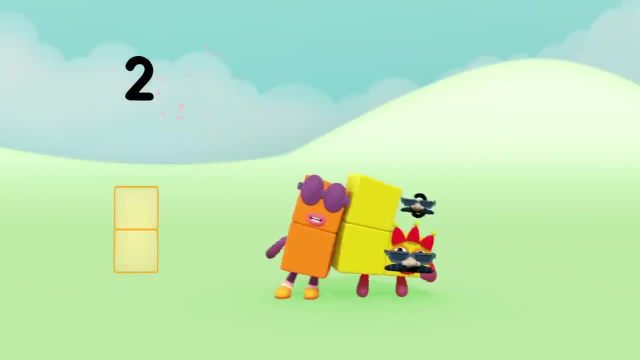 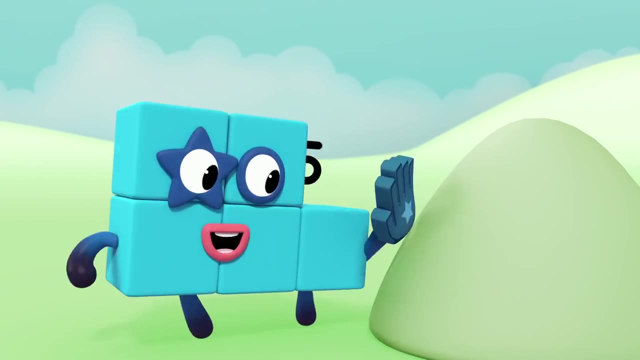 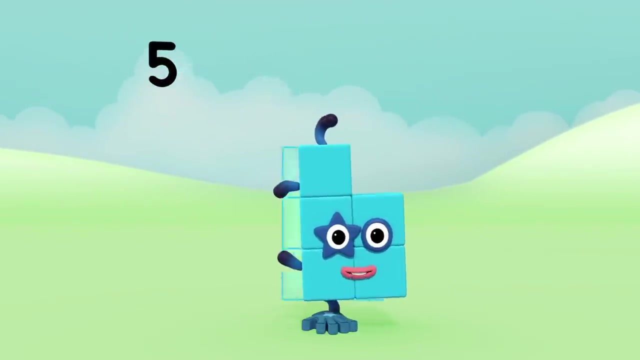 Two Plus three Equals Five. Ready or not here I come, Ready or not here I be, Find you two, find you three. Five minus three Equals two. A pair of pointing prints, Five found us, But but how? 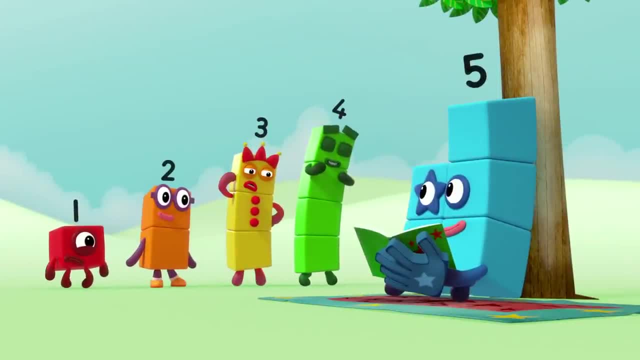 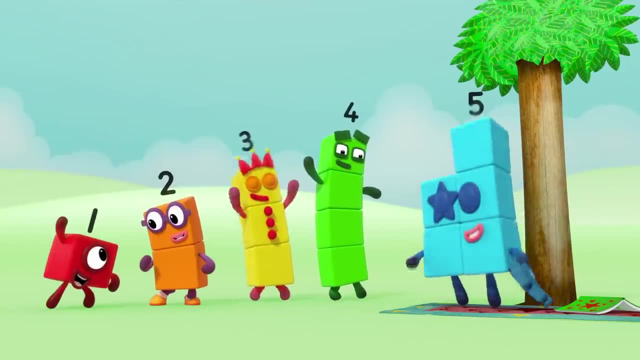 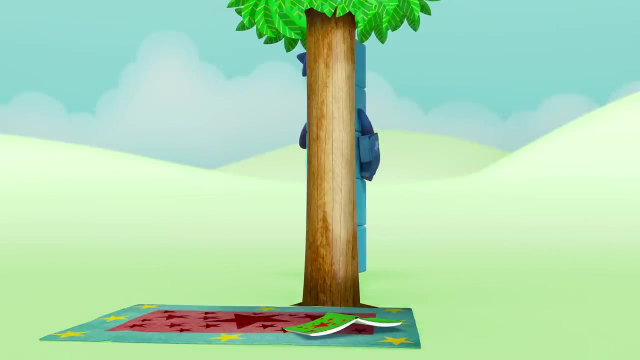 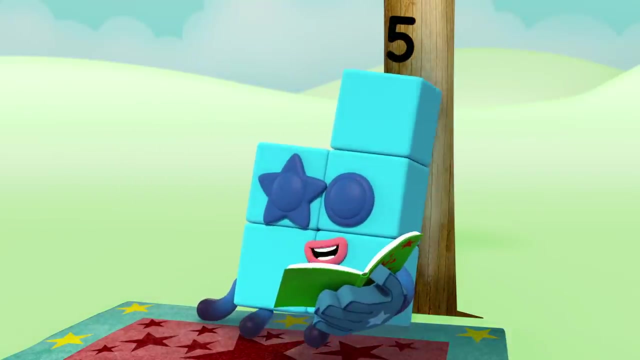 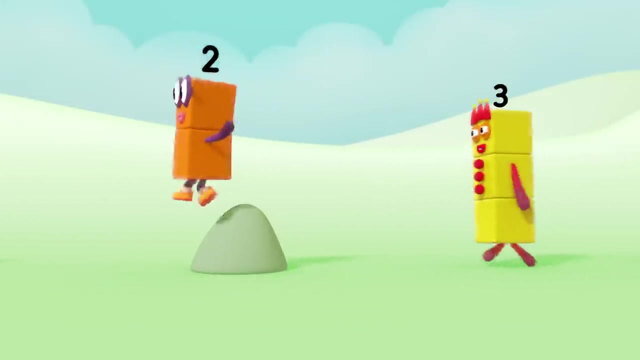 Five You're here. How did you Told you I was good. Now my turn to hide. Only day One, Two, Three, Four. Ready or not? five, here we come, Rock One Plus four. 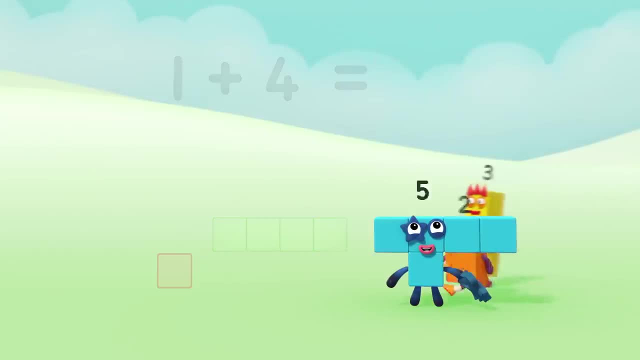 Equals Five, Found you. Amazing, Can you find me again? Five Minus four Equals one. Come on Rock. Three Plus two Equals Five Found you. Three Plus two Equals five Found you. 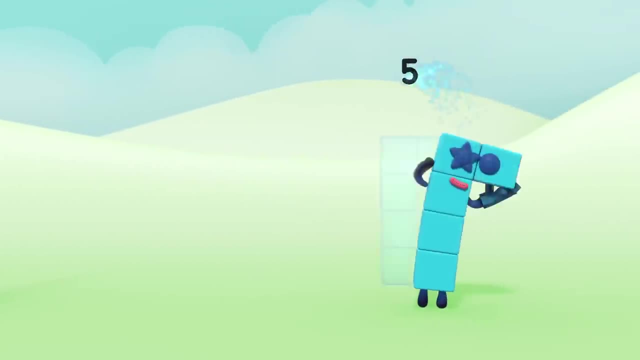 Five: Found you. Fantastic, Can you find me again? Five Minus two Equals three. Found you. Ha ha, ha ha. 5. Minus two Equals 3. Found you. Ha ha, ha, ha, Ha ha. 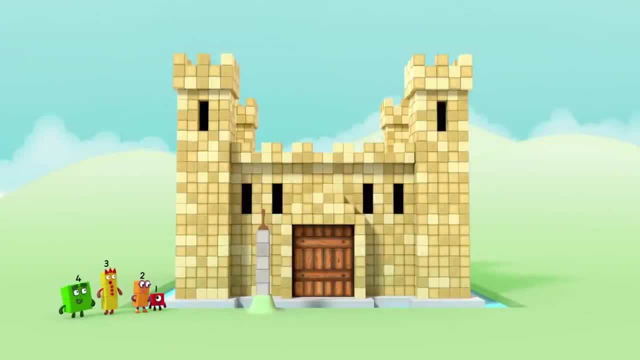 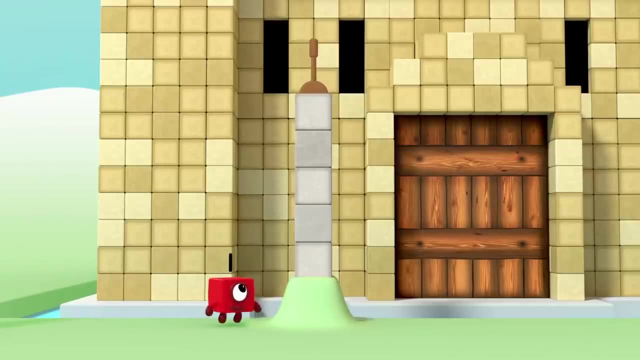 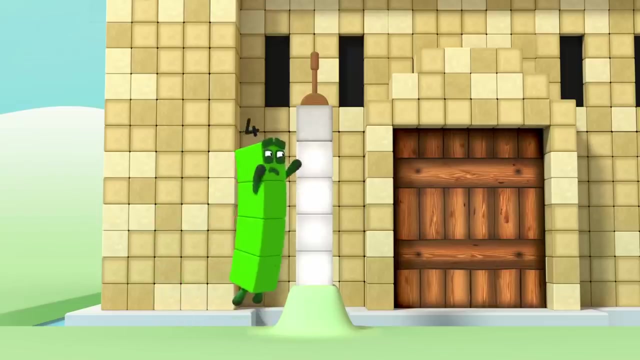 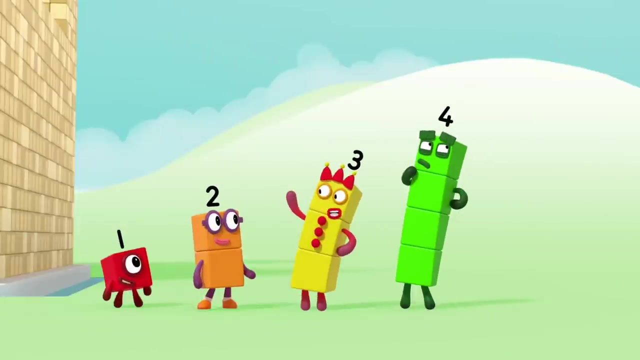 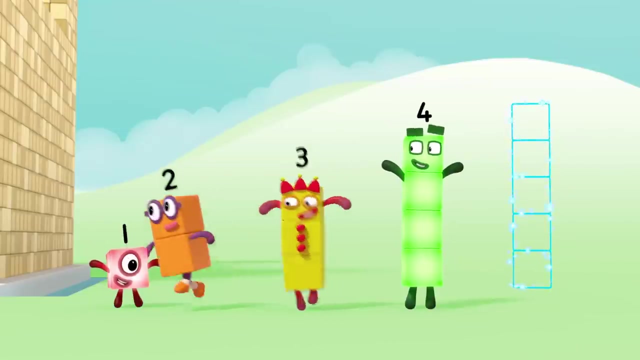 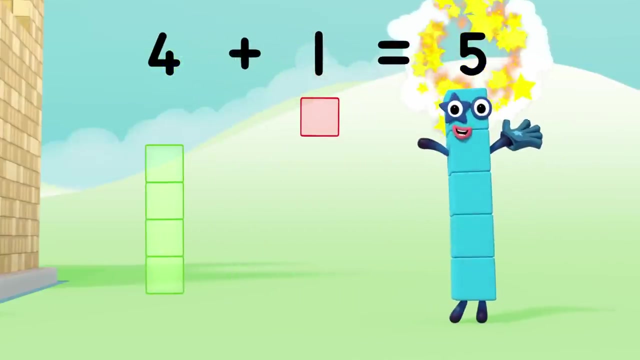 Great, I've found you Great. How do we get in? Maybe if we pull that handle. Oh, if only I was a little bit taller, Five's taller than four. So how do we get five? Four plus one equals five. 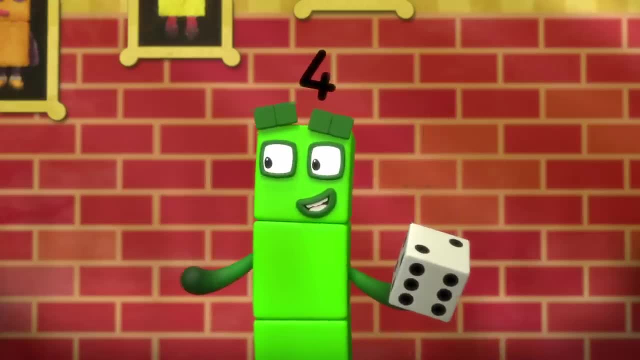 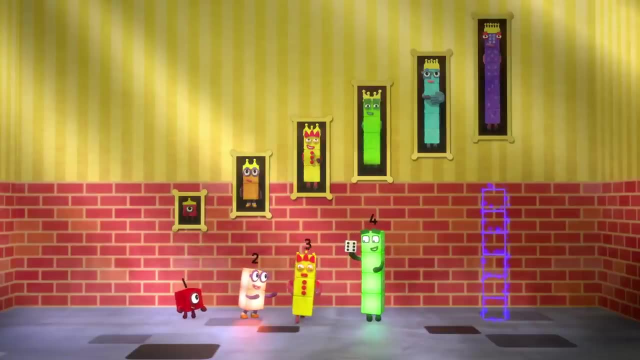 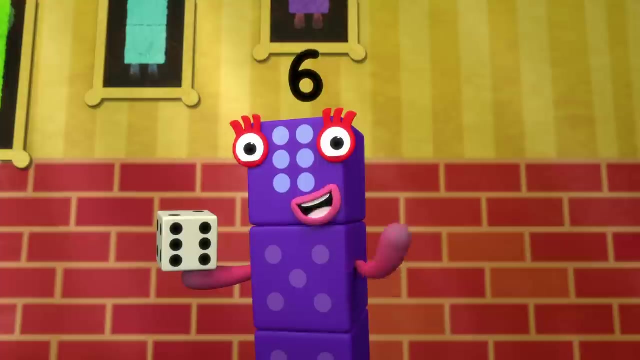 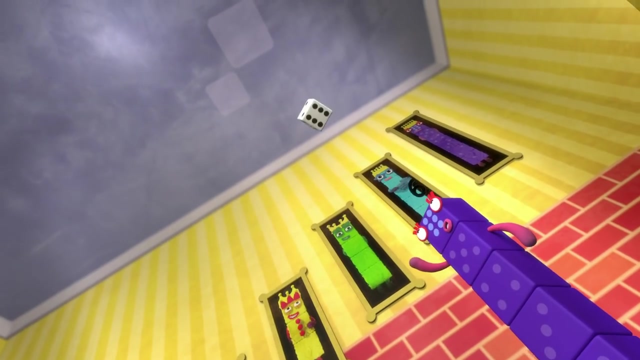 Dead end. Six is good with dice. How do we get six Four? Two plus two equals six. Hello friends, Here's my advice. It's time for me to roll the dice. Watch me give a little throw and you'll know which way to go. 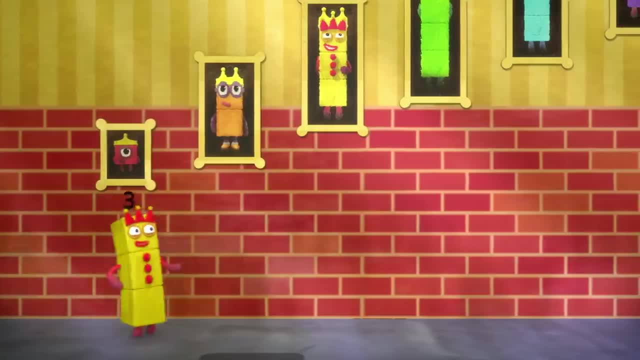 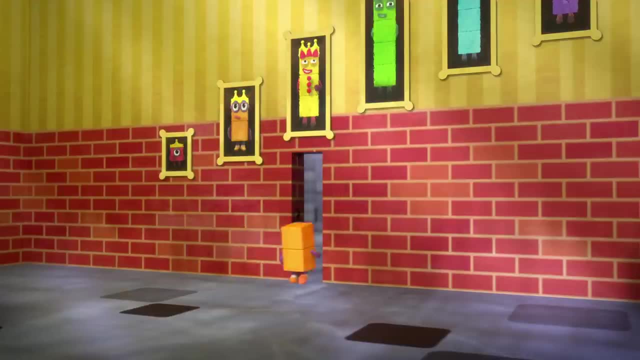 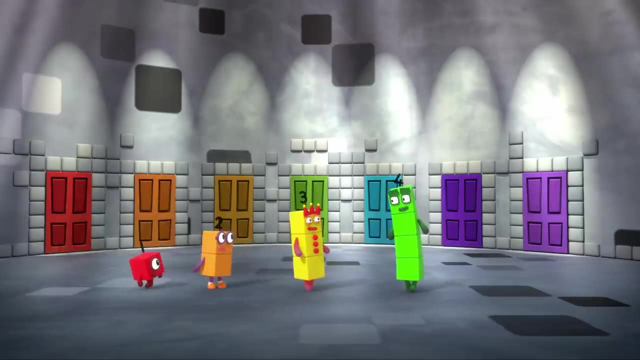 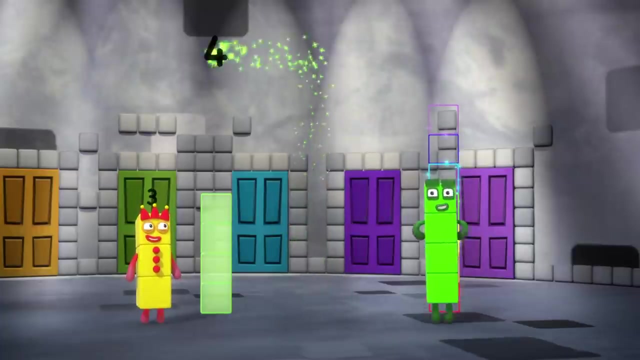 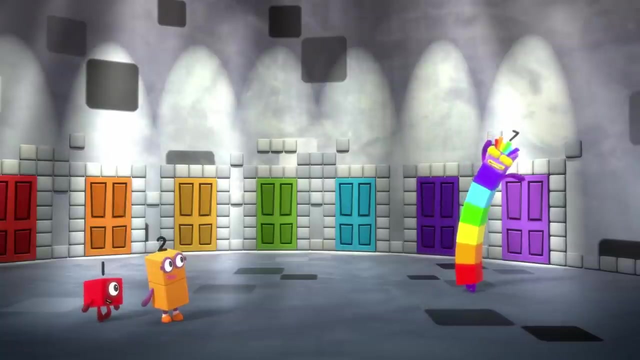 One, two, three, One, two, three. Follow me. Seven doors. Which door is right? Maybe seven can help. How do we get seven? Four Plus three Equals Seven. Oh, I feel lucky This way. 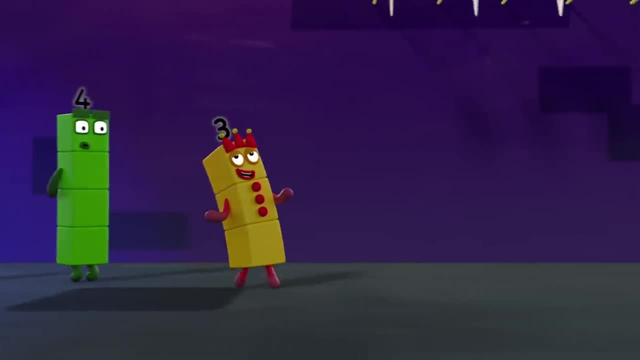 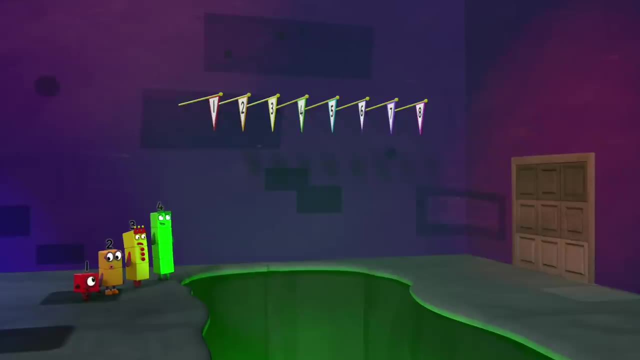 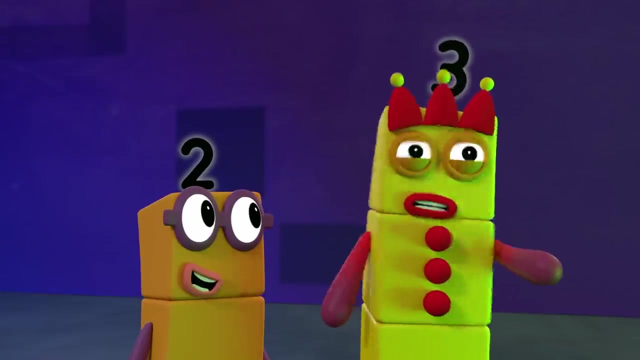 Easy peasy. Look at me-zy, We're stuck. No, we're not. We could swing from the flagpoles. We'd need someone with very long arms to stretch that high. Eight, How do we get eight? Four: 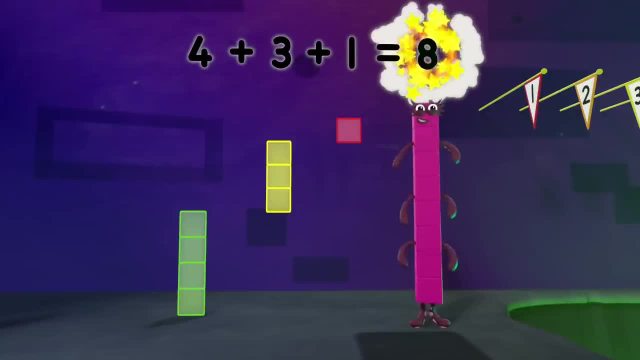 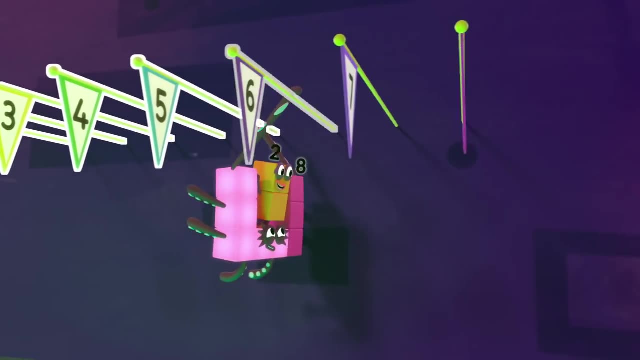 Plus three Plus one Equals Eight Octoblock swing. One, two, three, four, five, six, seven, eight, seven, eight. One, two, three, four, five, six, seven, eight. 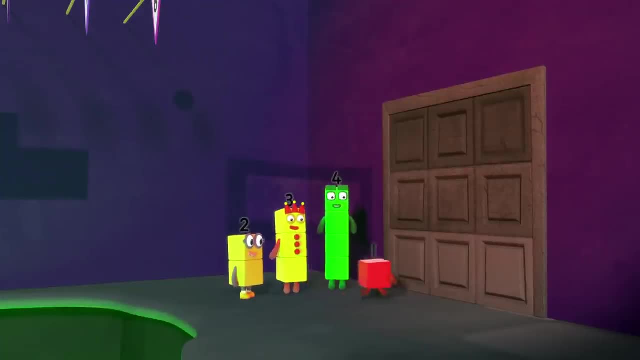 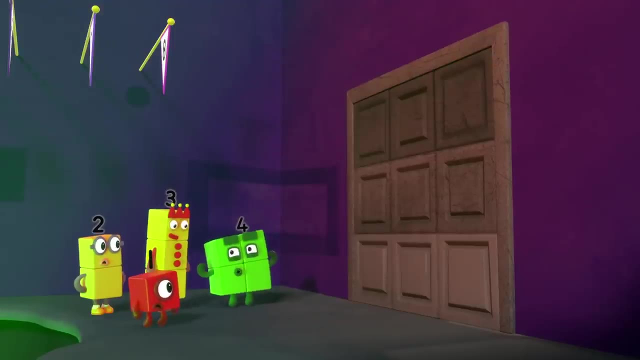 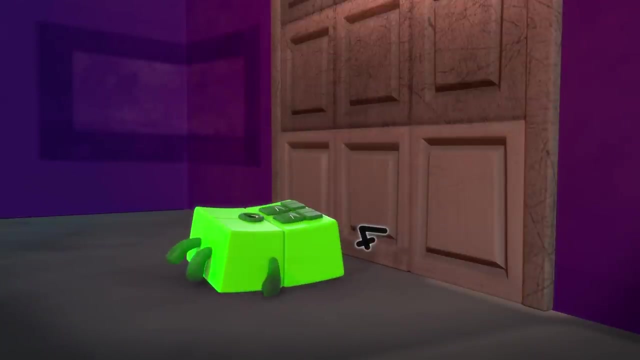 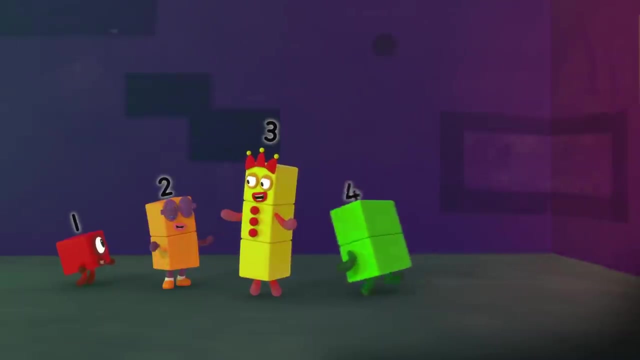 One, two, three, four, five, six, seven, eight. Swing, It's stuck. Squares are strong. Let me try. We need a bigger square. Nine. How do we get nine? Three, Six, Four? 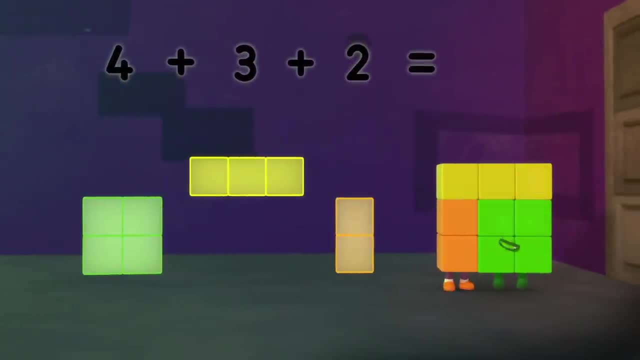 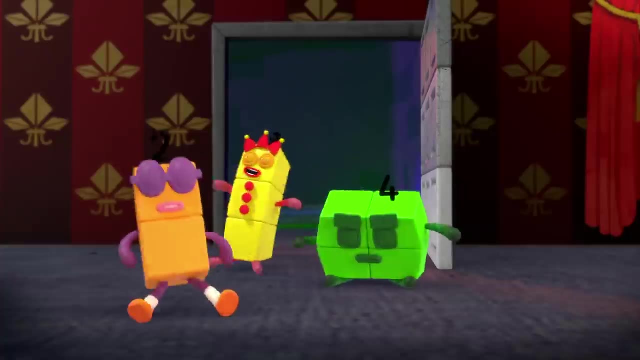 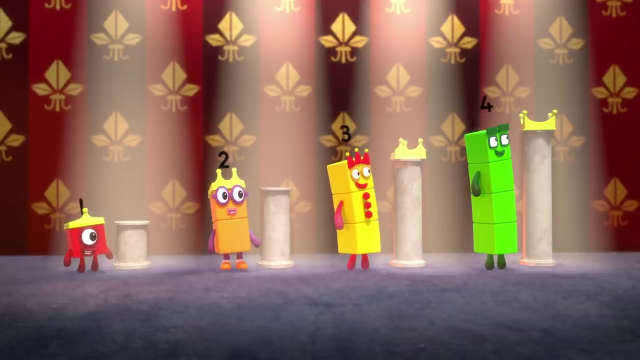 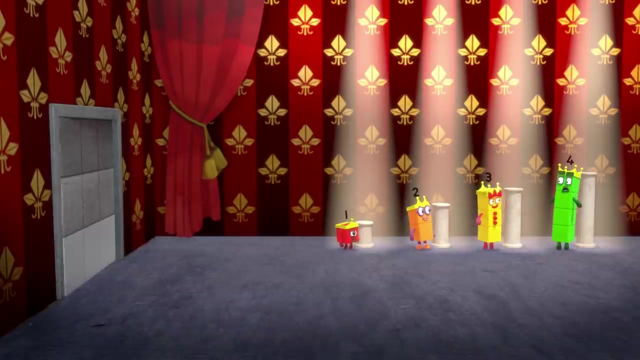 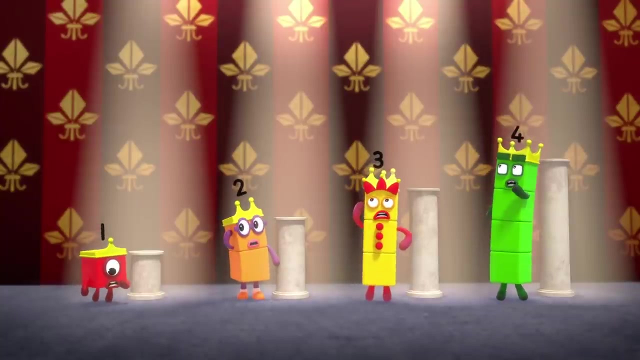 Plus three plus two equals nine. Thanks, One, two, three, four, Four crowns. Phew, Uh-oh. How are we going to get out? Oh, If ten was here we could rocket out through there. How do we make ten? 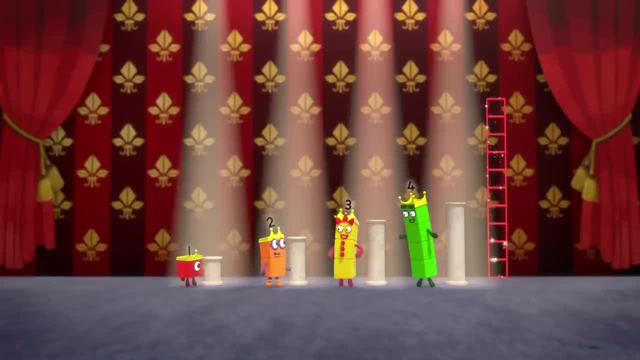 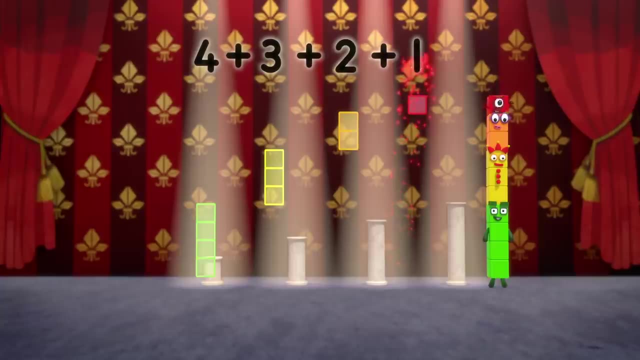 All together now, Four plus three plus two plus one, equals ten, Ten, nine, 10,, 11,, 12,, 13,, 14,, 15,, 16,, 17,, 18,, 19,, 20.. 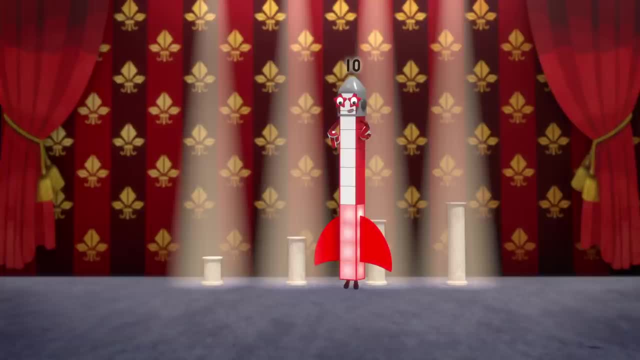 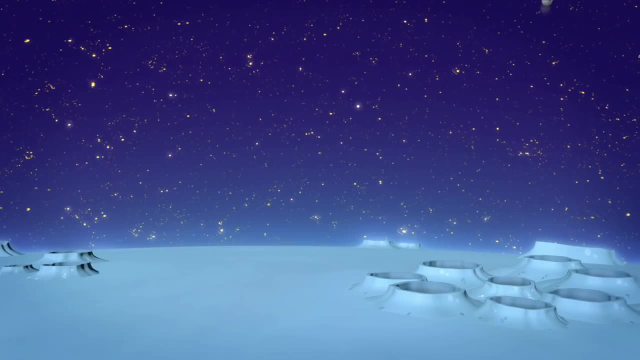 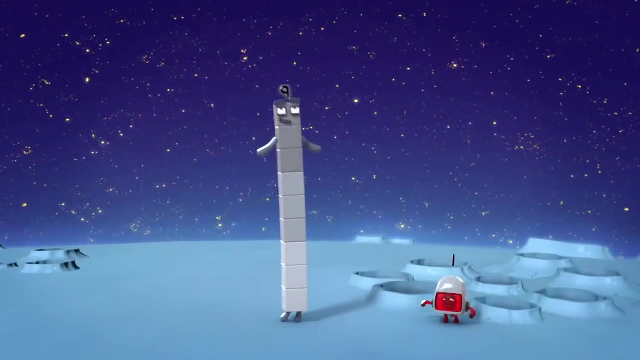 Nine, eight, seven, six, five, four, three, two. one Blast off Number ten up on the moon, And my friends will be here soon. Ten equals nine plus one. One small step for a number, One giant hop for number kind. 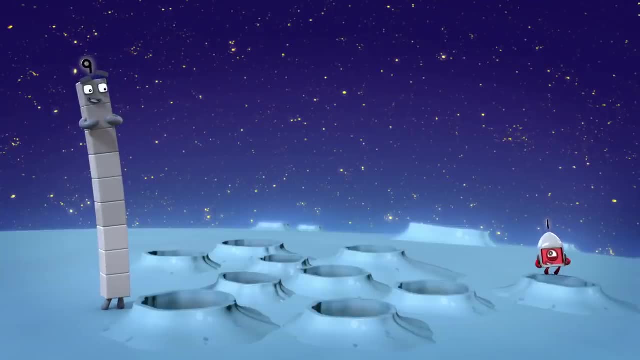 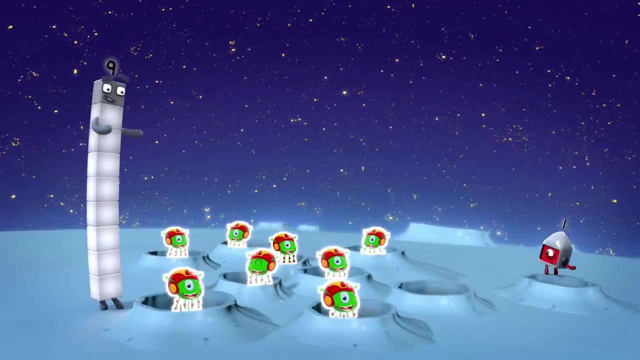 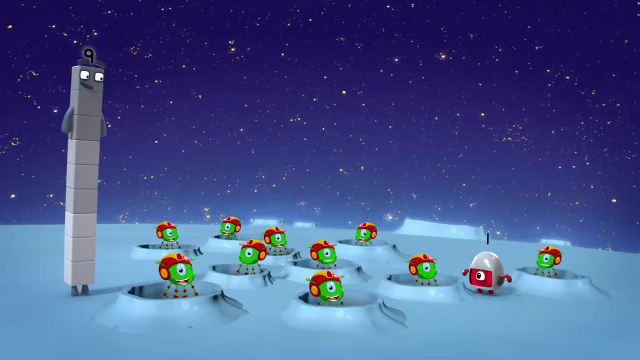 We're on the moon. We're on the moon. Nine And one. That was easy, This is fun. One, two, three, four, five, six, seven, eight, nine, Nine aliens, And one more is ten. 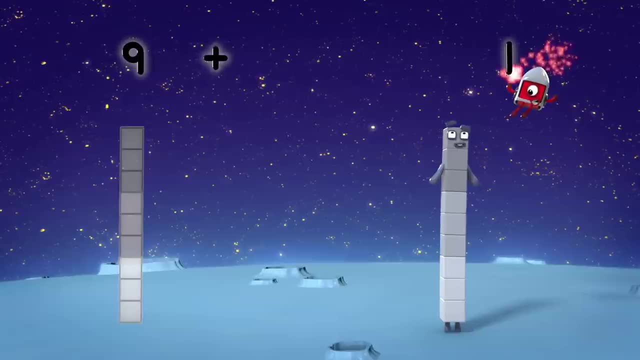 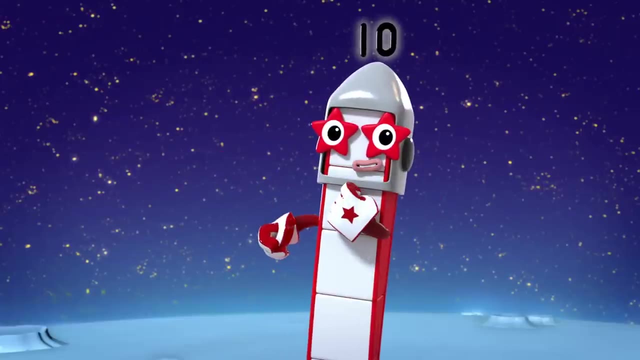 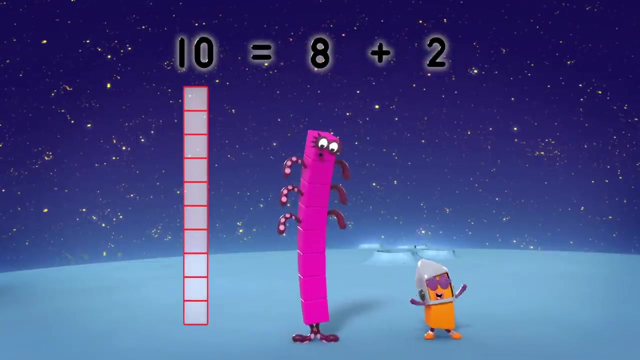 Whoa, Nine plus one equals ten. Number ten back on the moon. Two more friends will be here soon. Two more friends will be here soon. Two more friends will be here soon. Ten equals eight plus two. We're on the moon. 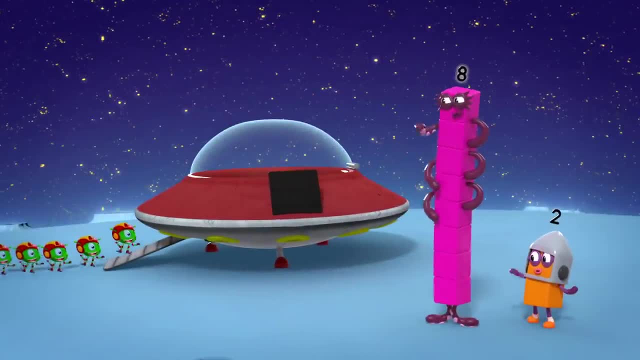 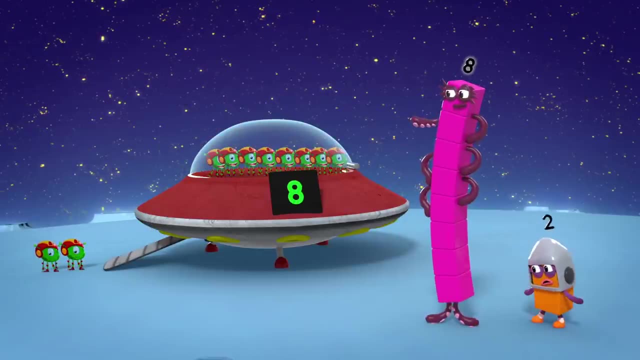 Eight And two. How did we get here? Haven't a clue? One, two, three, four, five, six, seven, eight, Eight aliens all heading home. Oh no, There's no room for those two. 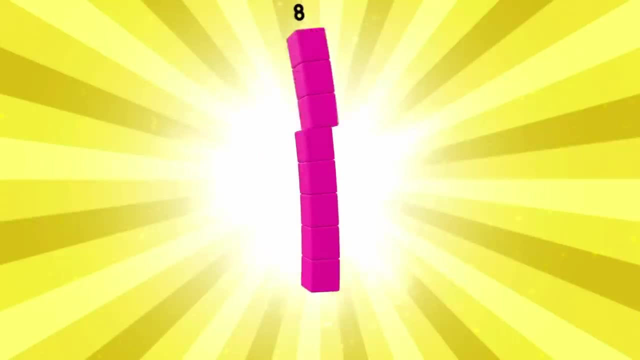 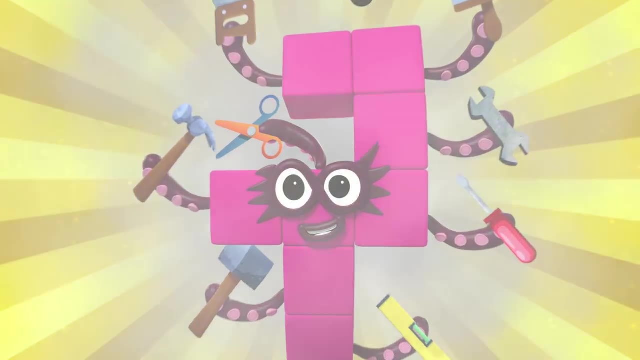 Never fear, Octoblock is here. Octoblock: Bill One: two, three, four, five, six, seven, eight. One, two, three, four, five, six, seven, eight. Bill Two: flying saucers. 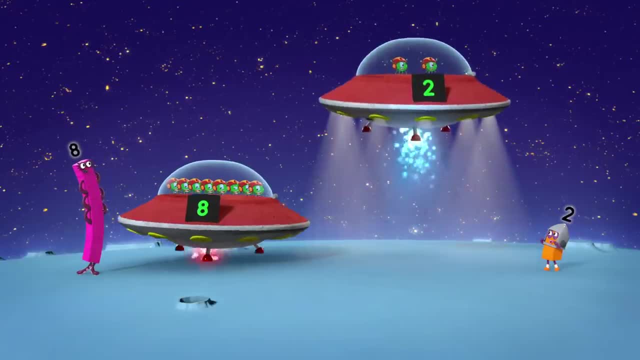 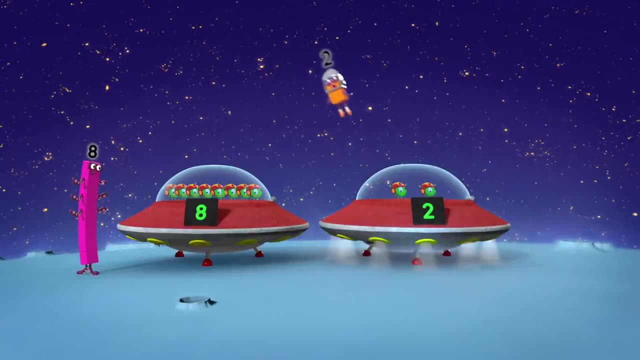 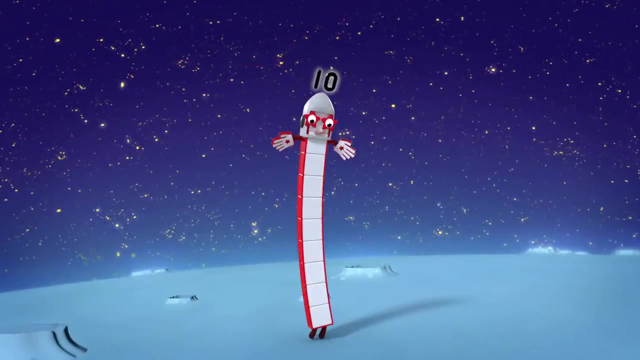 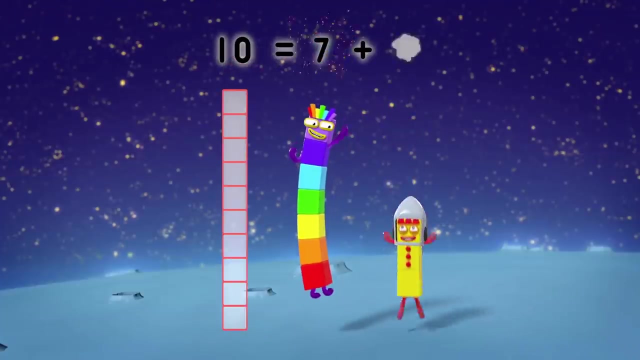 Good work. Oh, come back, It's not starting, Whoa. Eight plus two equals ten. Here I am. number ten. Time to make some friends again. Ten equals seven plus three. We're on the moon. Seven and three. 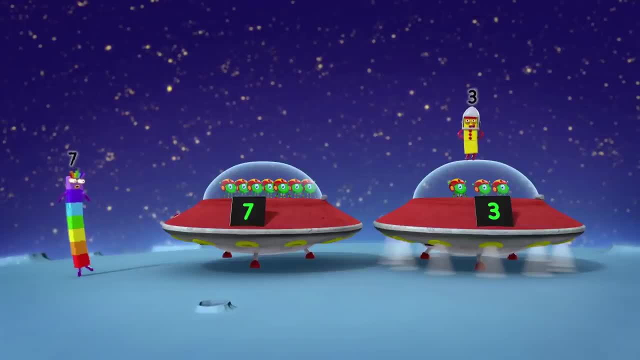 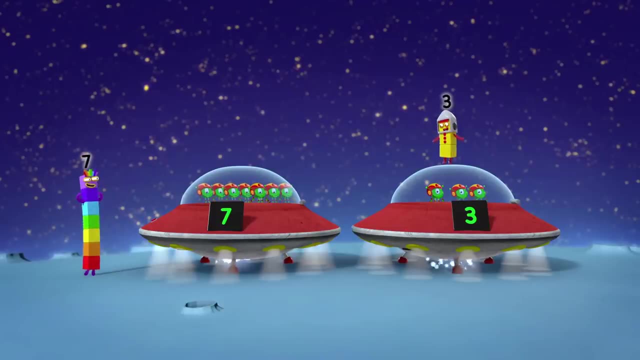 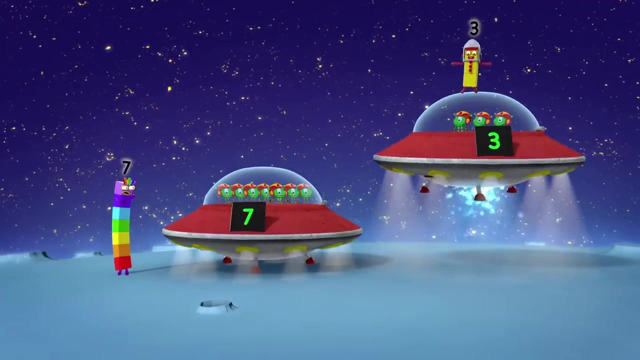 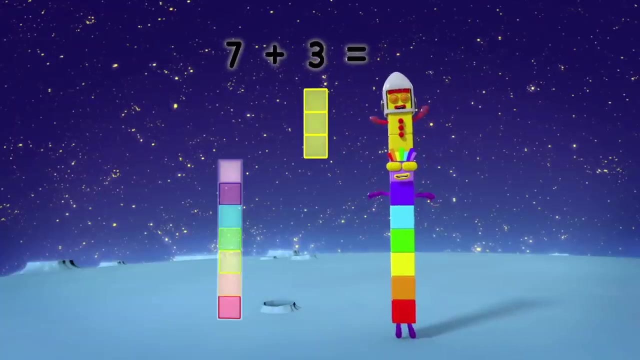 We're so lucky. Look at me, Woo-hoo, Look at that. There's the on button. That was lucky, Ready, steady, blast off. Whoa, Oh, it's too heavy. Seven plus three equals ten. It's ten again.